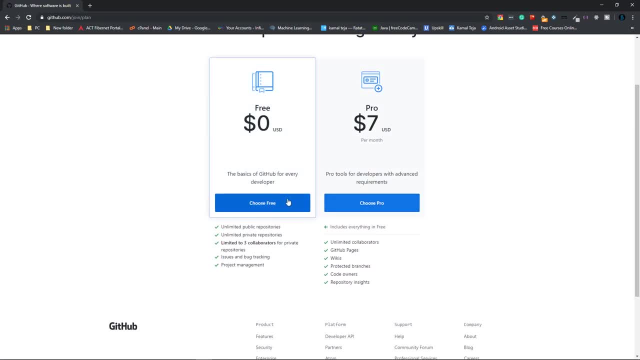 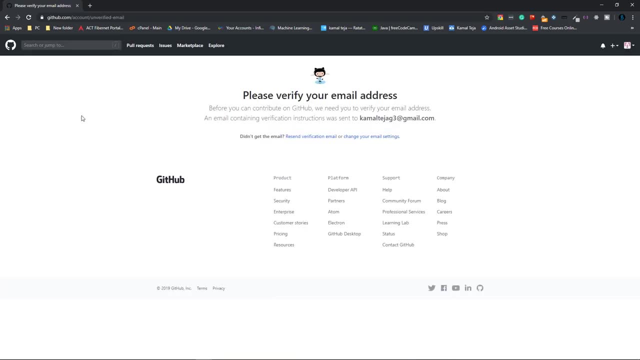 So there are actually two plans that you can choose from, but we are going to opt for the free plan, So click on that. Then they're going to ask a little bit about yourself. Then you can fill out that. Then they're going to send a verification option to your account. 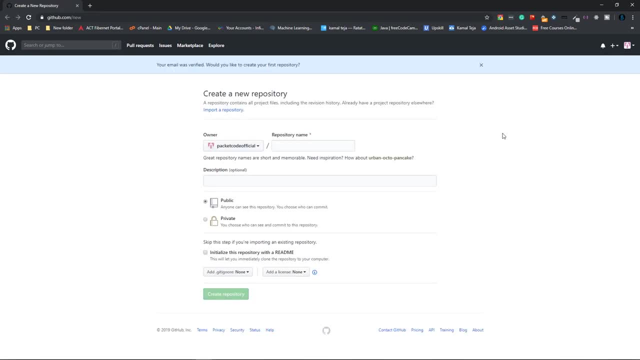 So please open your mail and verify that. So once you're done with the verification process, automatically you will be redirected to this page where you can actually create a new repository. So in GitHub sense, the repository is something like a folder where you can actually store. 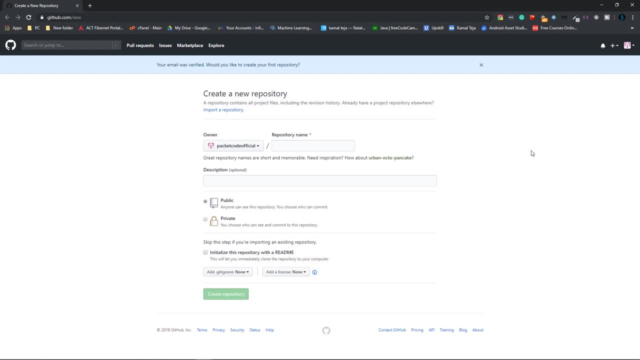 your files, So you can create multiple repositories for each of your individual projects and place the files regarding that particular project in that particular repository, And but the thing is that there can only be one hosting or one website URL That can be created from this GitHub account. 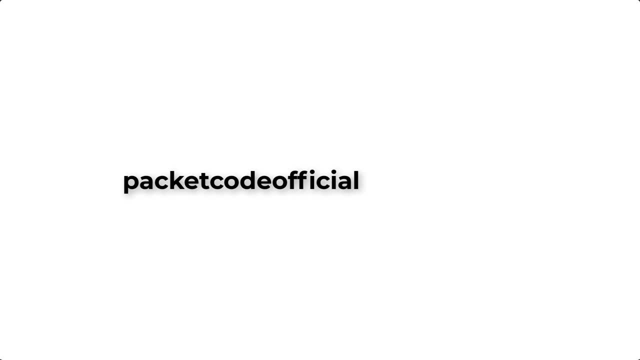 So for this GitHub account I have PacketCodeOfficial right, So for this I can only have a URL which is named as packetcodeofficialgithubio. That particular naming way is the only way that you can actually host the website, okay. 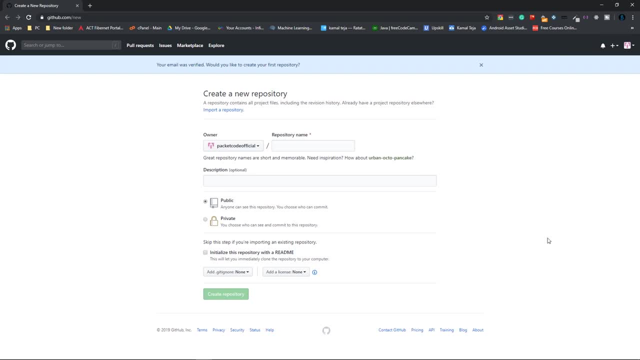 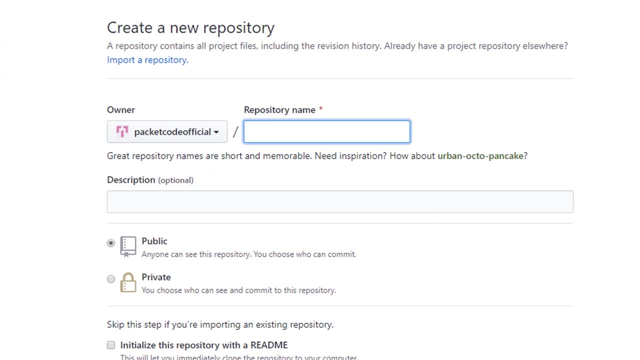 We can have multiple repositories, but all of those repositories will not be hosted. Only the particular repository with this particular name will be hosted. Okay, So let's name the repository as PacketCodeOfficial, So it's going to be PacketCodeOfficialgithubio. 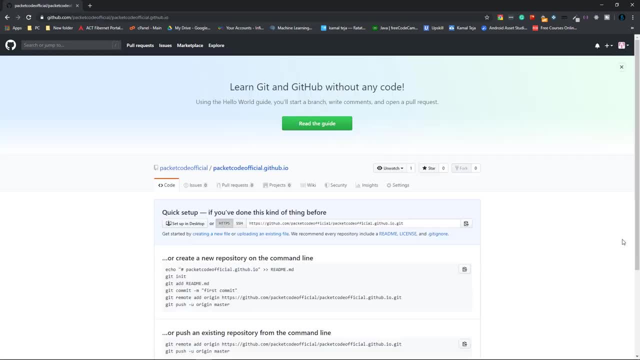 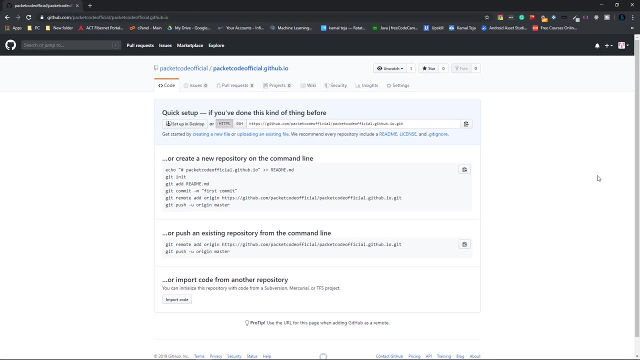 Then you can give a description if you want, or just click on create repository. So once you're done with that, you'll be redirected to this page where you can actually see that all those things is there, right? So this is actually used to upload the files to GitHub. 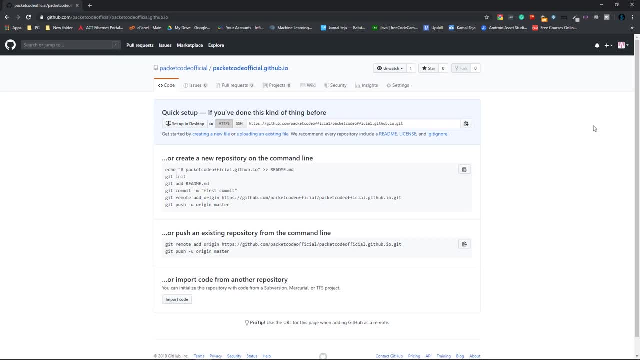 This might look difficult to you, but it's actually quite easy. So to upload files to a GitHub account, there's actually two ways that you can do it. The first one is using the git command line, So first you have to download the git command line. 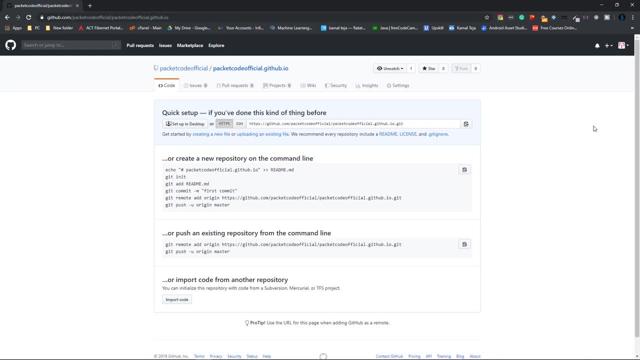 Like the version controller git on your computer. then you have to open the command line and type in all of these commands. then that will be uploaded or there's another way you can do that. So they have created an application, a desktop application, known as GitHub desktop, through. 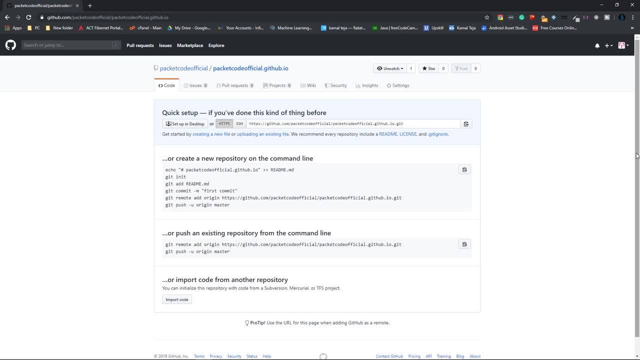 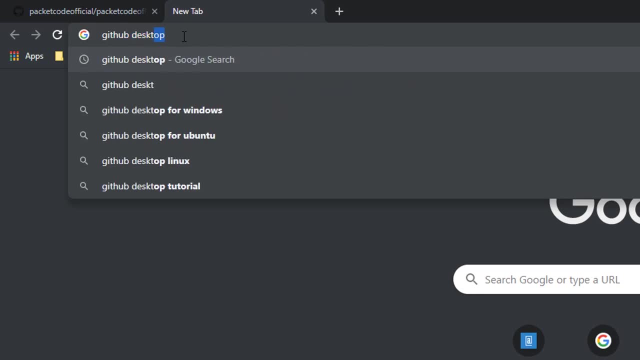 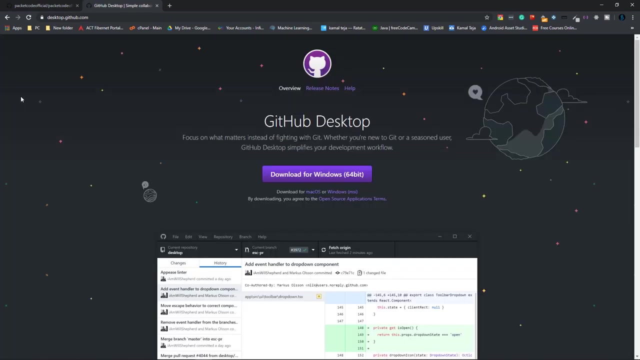 which you can actually upload the files in the same way, but it has more of a user interactive interface. Okay, So open a new tab and search for GitHub desktop. Then open the first link. So this GitHub desktop is similar to the original version control of git, but it has more of. 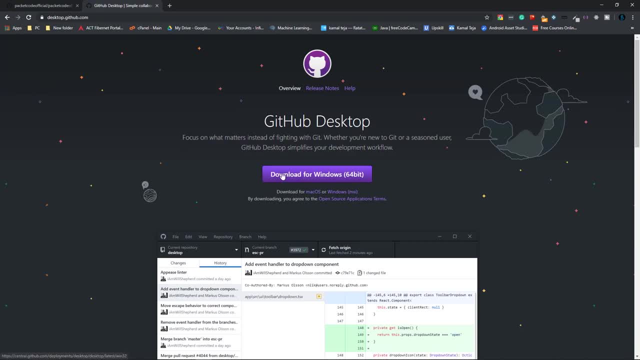 that, as I mentioned that user interface. Okay, So click on download. but if you're more of a techie guy, then I suggest you to use the version controller git itself, as that is going to be more versatile for you than get this GitHub desktop. 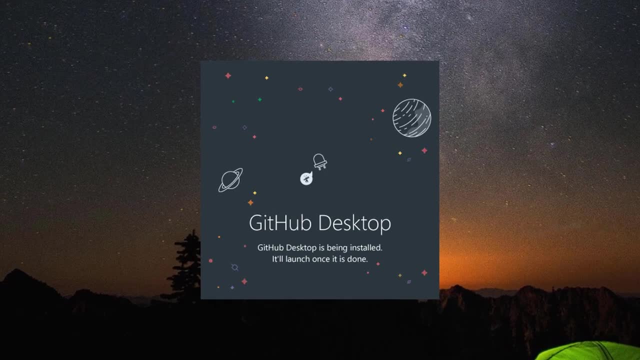 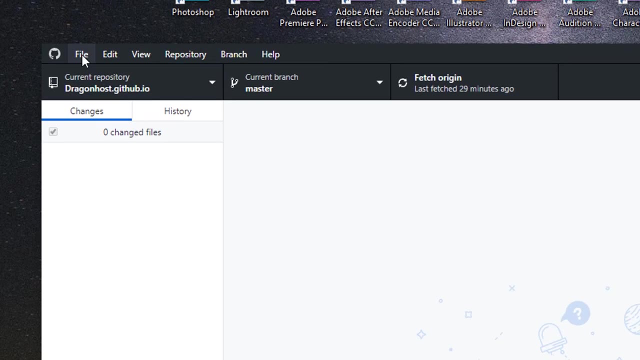 Okay, And once you're done downloading, click on the download icon and this should pop up. So once you're done installing it, you'll have an interface that looks something similar to this. So there you will have an option for file. Click on file and you'll have the option for clone repository right. 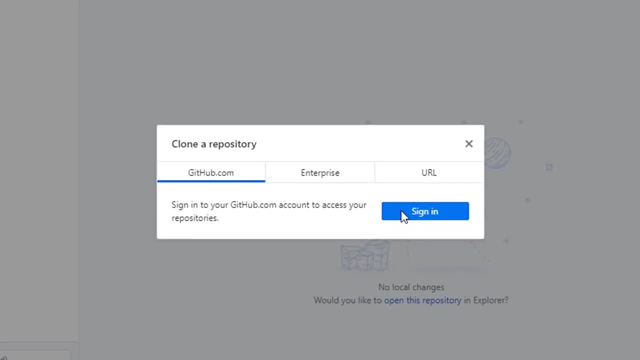 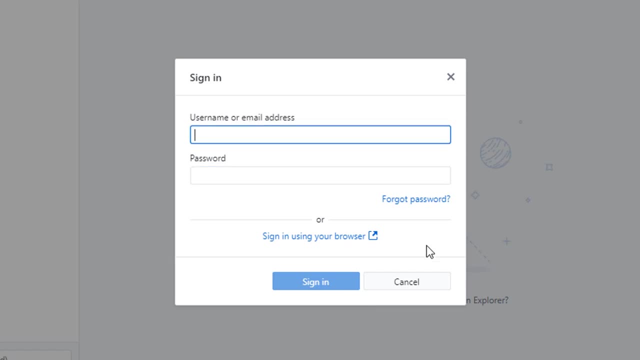 So click on that, Then you'll be prompted with signing a sign in option. Click on sign in, then give the username and the password for that GitHub account that he had created just now, or you can sign in using your browser. So I'm going to click on that automatically. 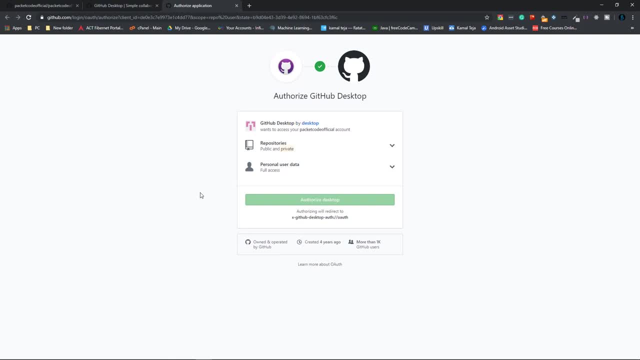 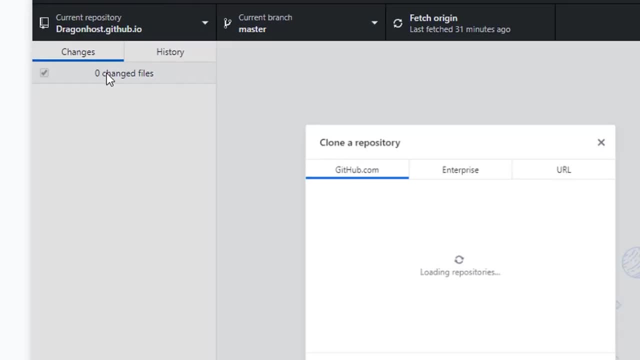 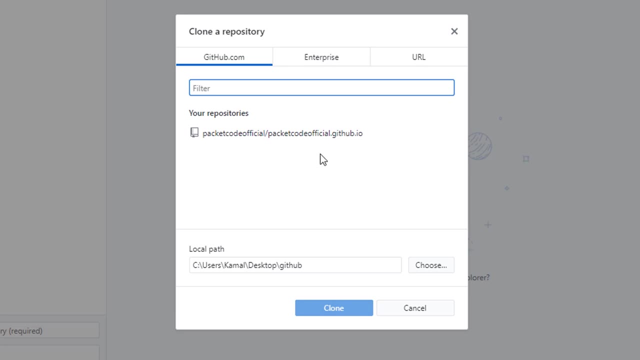 It's going to open my browser and ask for my permissions. Click on authorize desktop. So once you're done signing in, then click on file and clone repository Once again. now you'll have the option for packetcode- official slash- packetcodeofficialgithubio. 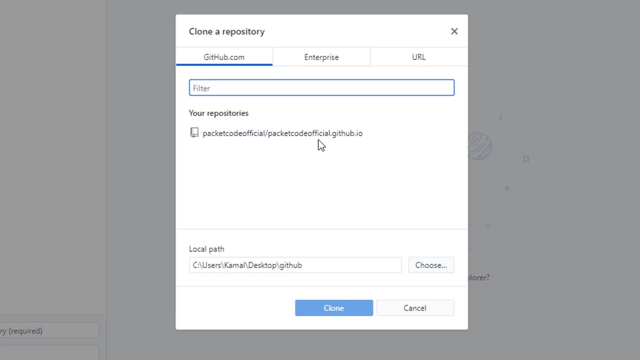 So that's the deposit that have created. You'll have your own repository, So click on that, and then at the bottom you have the option for selecting where you want to create that particular file. So when you have to choose that, okay, so choose that particular location where you. 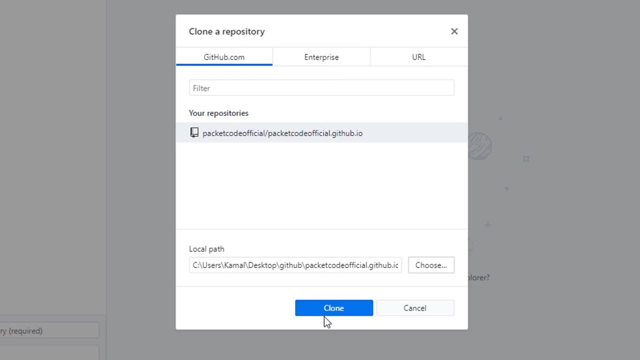 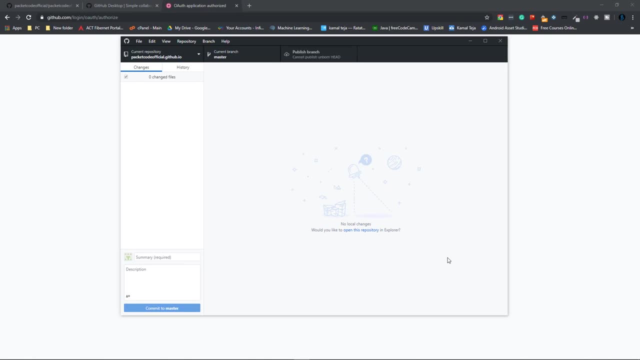 want it to happen And once you're done choosing it, click on clone And that is going to create a folder With the name of GitHub in the place where you have given the location. So for mine I have given it as the desktop. 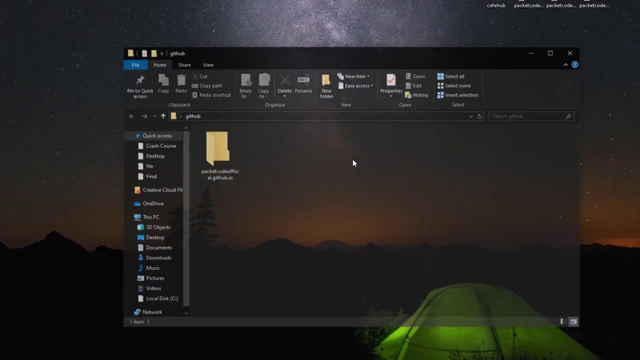 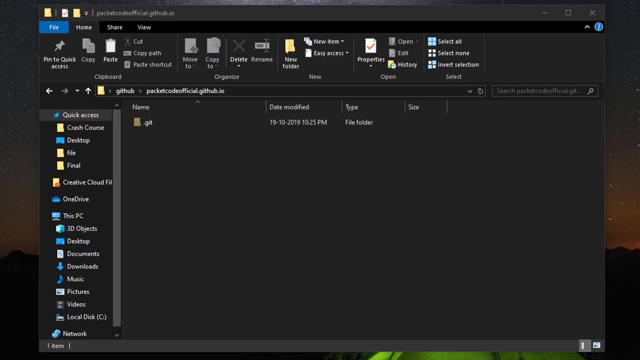 So it's going to create a folder called has GitHub for me on my desktop And in that it's going to have that particular folder or repository in my GitHub account. So open that and open the folder where you have the files that you want to upload. 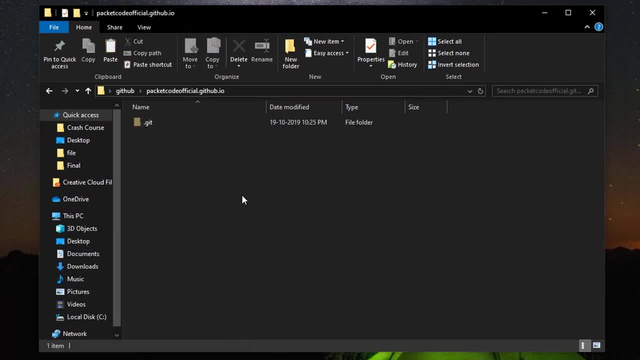 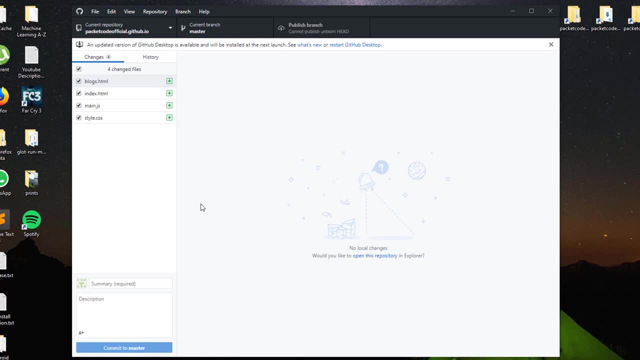 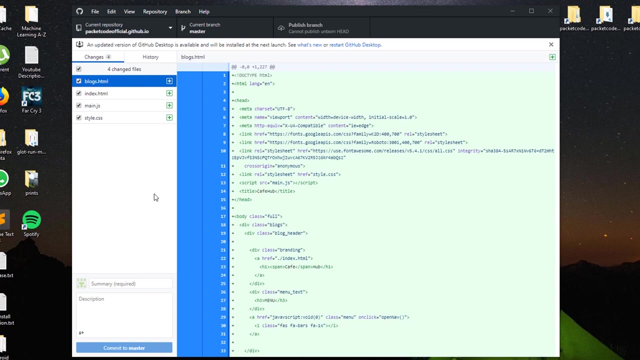 Then copy that files. okay, copy that and paste that in this particular folder And once you're done with that, then automatically, if you open the GitHub desktop icon, you'll see that all the files have been added And you can see that it's showing me four changed files. 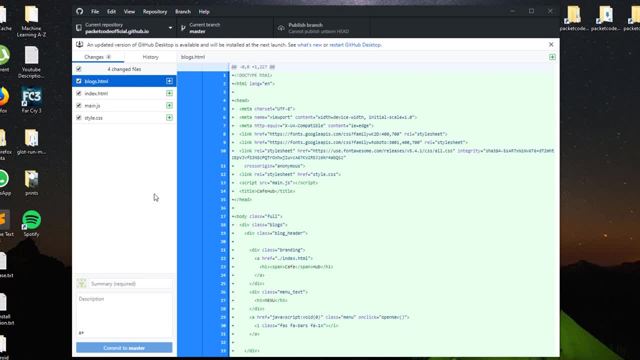 So the process of me adding that files into this folder has been seen by the GitHub desktop and it is prompting me that you have to update your repository. So now I'm going to give a summary. So let's say I'm going to give it as added new files. 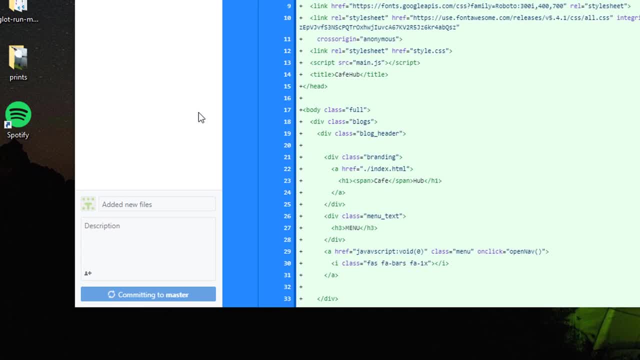 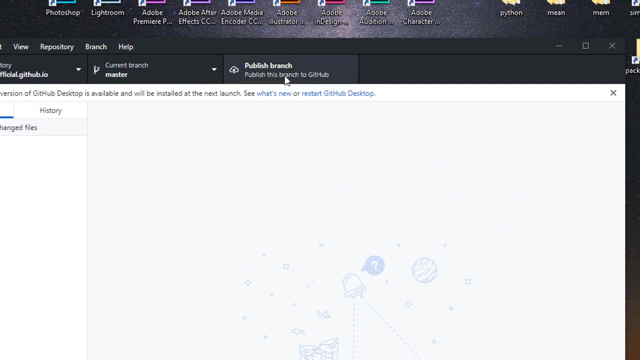 And once you're done with the summary, click on commit to master, So that is going to link to your repository online And once it's done it's going to show an option for publish branch. So click on that So it's going to publish or place these files in your repository. 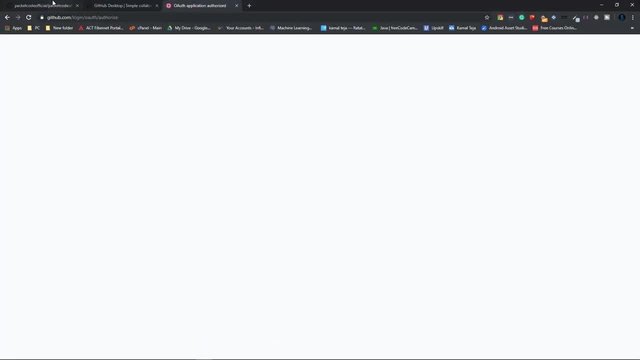 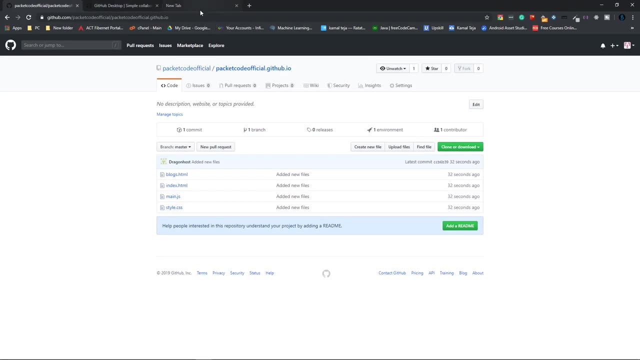 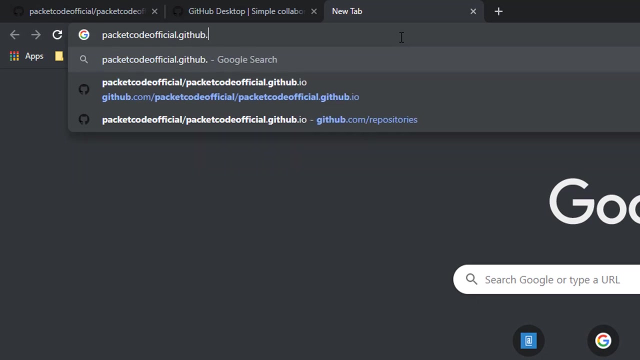 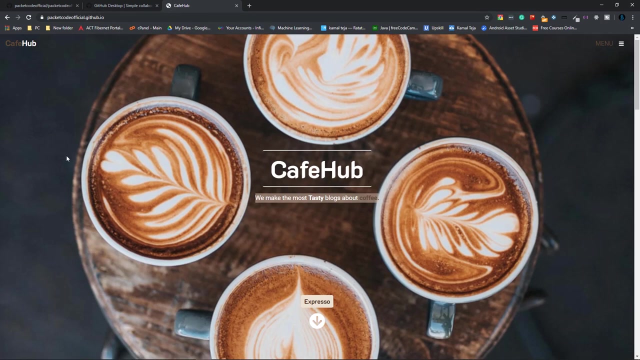 So once that is done, open your browser and go to your GitHub account. Then refresh the page automatically. you see the files here. So now what you can do is open a new tab and search for packet code- official dot github- And once you click that, automatically it's going to open the file that I have created. 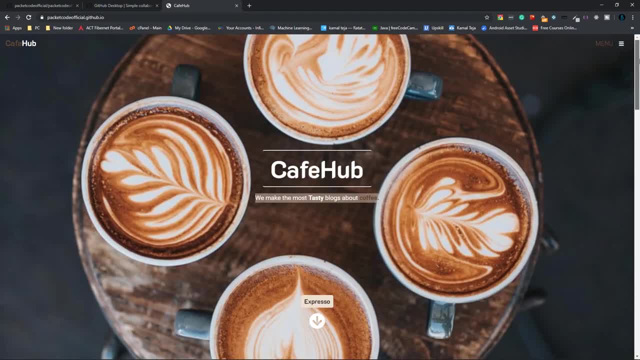 So this is the index piece that I have created. So this is my project and it's going to show that. So in this way, you can actually host static websites on GitHub for free. And for those of you who have seen this till the end, I have a special tip for you. 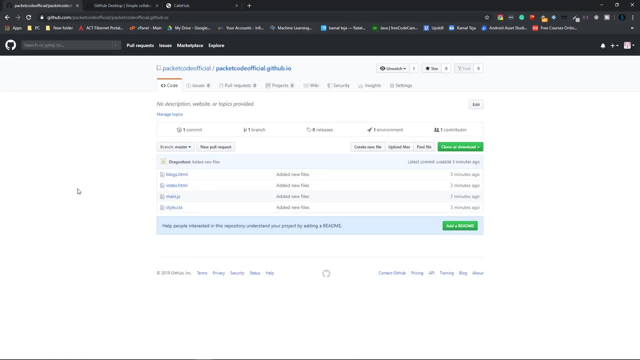 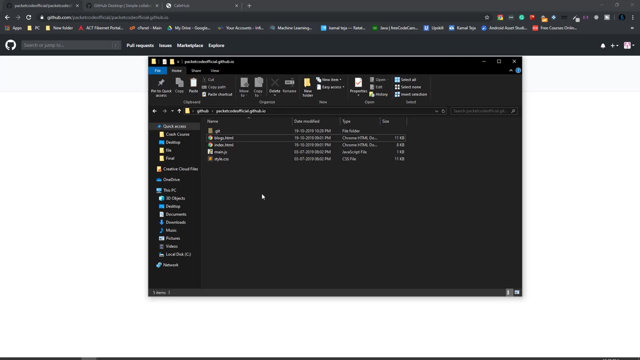 So, in your GitHub repository, do one thing. Instead of uploading the files directly, what you can do is go to your folder in your desktop. You have this right Packet code: official github I owe in that, instead of placing the files directly, create a folder. 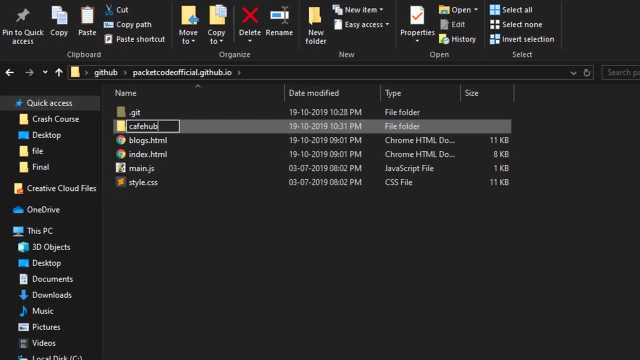 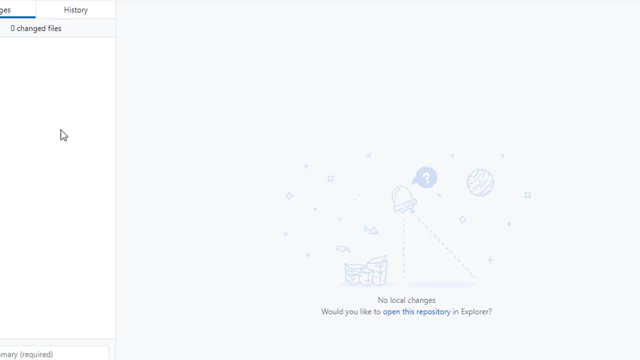 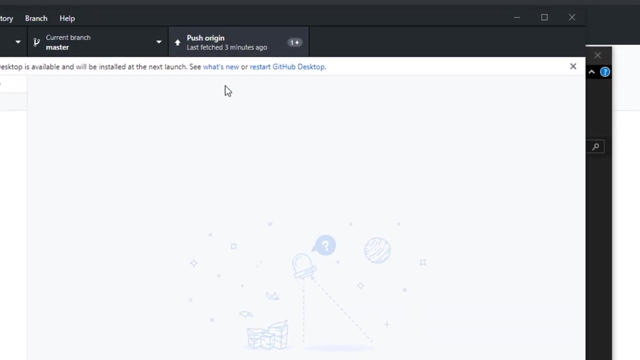 Okay, so let's name my folder as cafe hub and place these files, these particular files, in that folder and then go to a desktop version of that, Then type in a new summary. it's going to be updated. commit to master, then push origin. 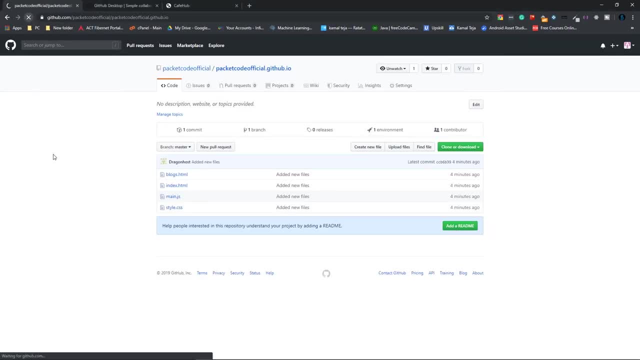 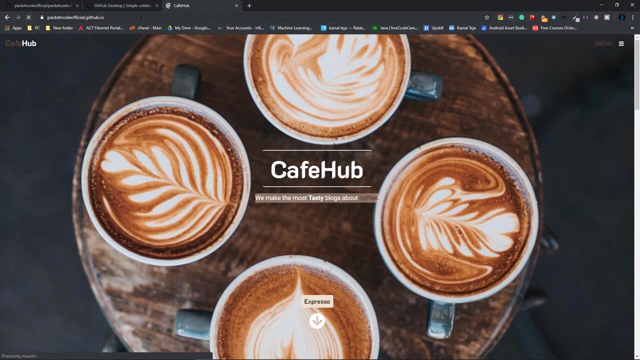 Once you're done with that, close that and refresh the page. automatically. you'll have the folder called cafe hub. So in my official GitHub page, what I'll do is, instead of typing it as packet code githubofficialcom, I'm going to give a slash and give cafe hub, and that is going to open the same page. 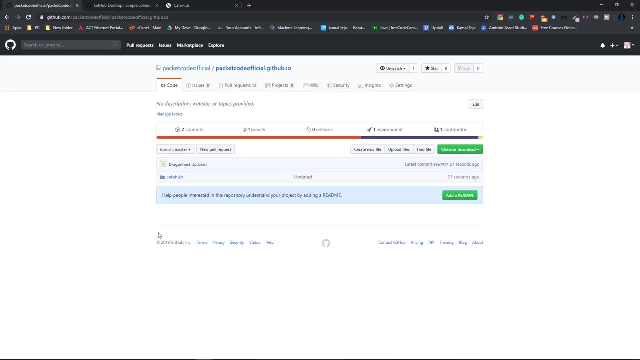 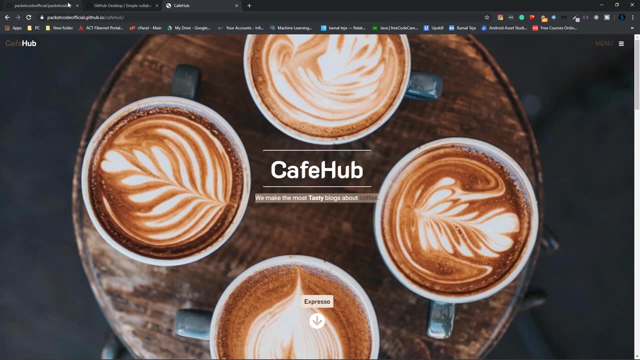 Okay. So by this trick you can actually upload multiple files and instead of giving it as directly packet code officialio, you can give it slash your particular project name. So in this way you can host multiple number of static websites on your own GitHub account. 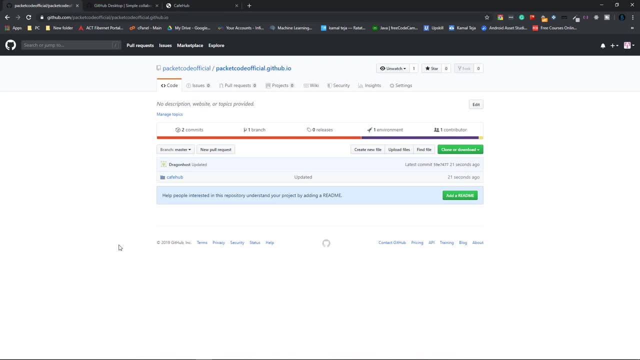 for free. Okay, So that's the tip I have for you guys. Thanks so much for watching, guys, And if you haven't subscribed to this channel yet, then please do subscribe. And this is Kamal signing off. See you in the next video.